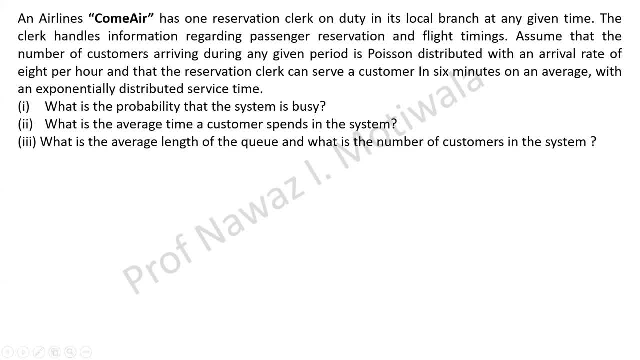 Good afternoon. let us start with today's session, Okay, so let us start with the questions. Again, I want your attention, as I already told, that if you make one mistake- or let us say two mistakes- one will be the arrival time and one will be the service time. If you make the mistake in fetching this two data, the entire problem will go wrong. you will be getting zero instead of 10. And if you get it correctly, there is 99% chance that you will get full 10 marks, because rest all is just application of formula. 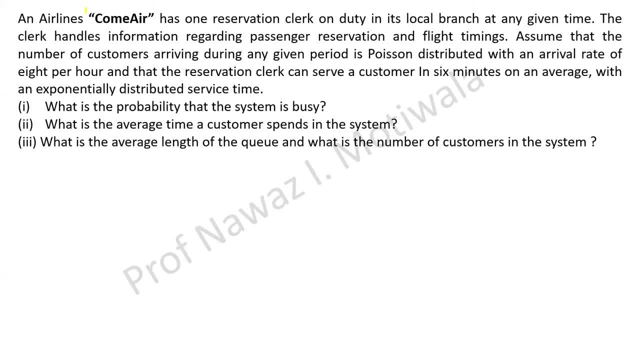 Okay, so let us start with the question. Airlines, let us say I have named it. come air has one reservation clock on duty in its local branch at any given time. Okay, the clerk handles information regarding passenger reservation and flight timings. Okay, 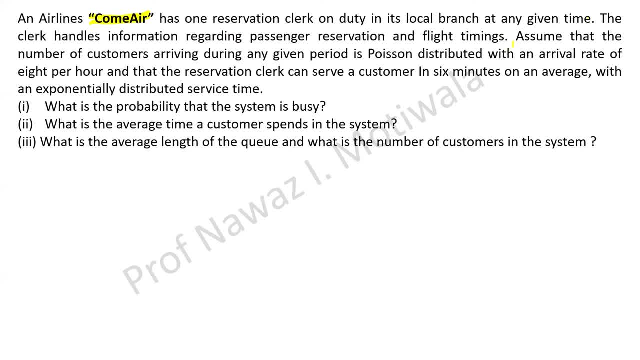 he is handling something regarding reservation and flight timings. Assume that the number of customers- this is the important thing- Assume that the number of customers arriving arriving, so what will be there? What will we use for arriving? Lambda. Okay, so we are talking about arriving, so we will be using lambda. Arriving during any given period is poison distribution, which we have already seen. it will be poisonly distributed with an arrival rate: arrival rate of 8,000.. 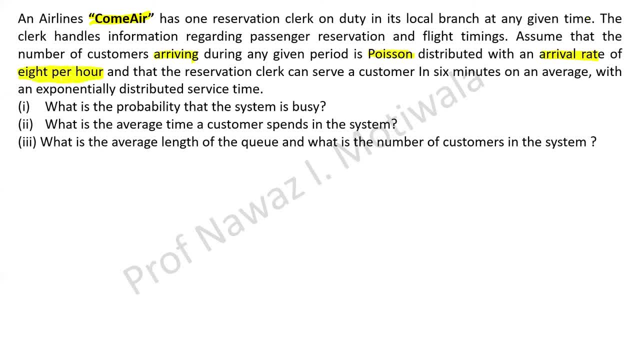 8 per hour. So already we are given 8 per hour. So can I write: lambda is equal to 8? Directly I can write: lambda is equal to 8.. So lambda is equal to 8 because directly we have been told 8 per hour and we also need lambda in the answer per hour. I forgot to write here It will be 8 per hour, So the entire unit will be lambda is equal to 8 per hour. Then, okay, let us go further And the reservation clerk can serve a customer. 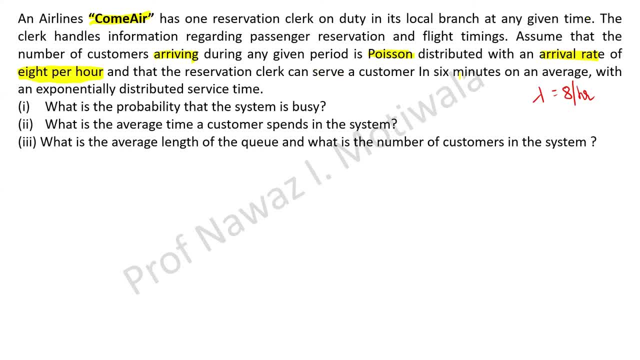 What is its service time? Can serve a customer in 6 minutes on an average. So can I write: mu is equal to 6?? Yes, sir. Yes, Okay, Those who have given answers as yes are wrong. Look, I told you earlier what should be the unit. Unit should be per hour, How many customers are served per hour, And here it is given in 6 minutes on an average. So first of all you can see from here: there is a minute given here. 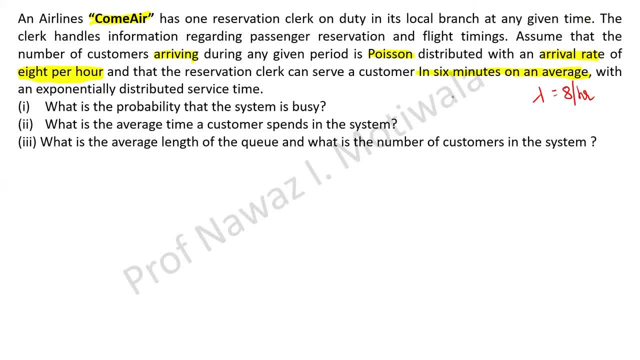 You need it in hours, So you cannot write directly. mu is equal to 6.. Now we will think a little about this. What can happen? Look now, logically, tell me what I told you, What I explained about lambda and mu. Lambda is how many customers. What is lambda? How many customers arrive per hour? 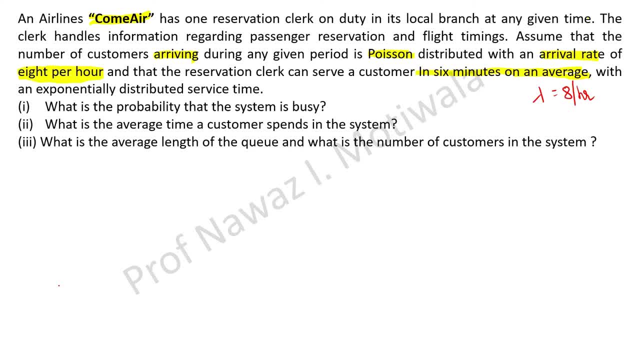 Let us say 11 to 12.. Between 11 to 12, an average of 8% is coming, Okay. Between 12 to 1, an average of 8% is coming. 8 persons, Okay. So that is the rate of arrival And what is the rate of service. What I told It is how many of them are served per hour. How many people got service in an hour, Okay. So now what is being said here? A reservation clerk serve a customer. It takes 6 minutes to serve a customer, Okay. One customer is served in 6 minutes. So how many customers he can serve in one hour? 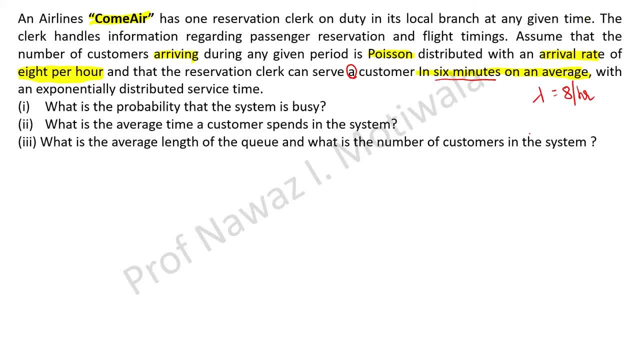 10.. So that will be my mu, So I will write: mu is equal to 10 per hour, So this will become my service rate. So now any doubts in lambda and mu? This was the important thing which I want to explain. 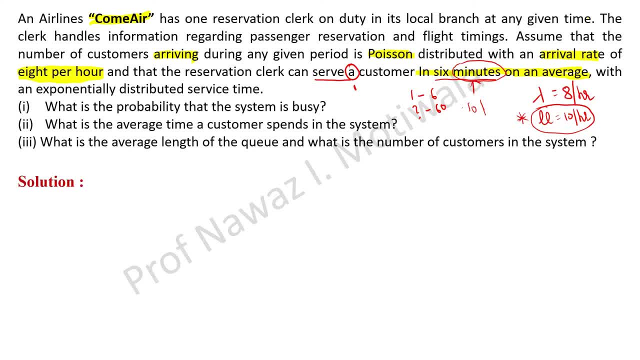 Lambda and mu, No doubt? Okay, No, sir. So solution: Lambda is 8 per hour Already, given I took out the service rate of 10 per hour And what we are required to find. Okay, This is also important. First you need to understand what to find. Okay, Let us go for the question. 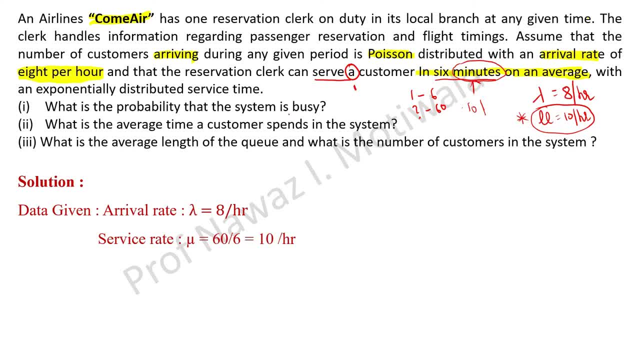 What is the probability that the system is busy? The problem is what I need to find out: Utilization factor. Yes, it will be a utilization factor. How much time will that service be utilized? And if you ask an IDLE, we will discuss that too. If you ask IDLE, it will be 1 minus. server is busy. So here I want to find out the traffic intensity or utilization factor. that is rho, And maybe its formula is lambda by mu. You check it, Okay. Next, 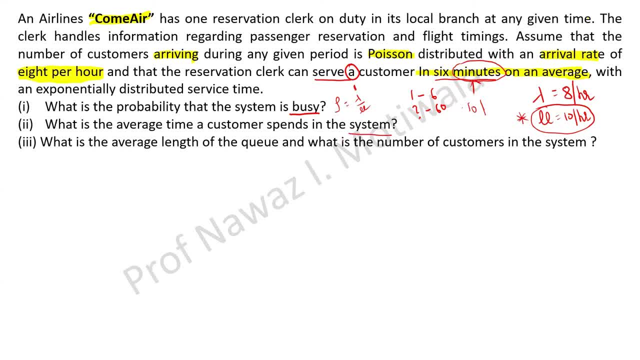 What is the average time a customer spends in the system? So what I will write here, What I need to find. First of all, the time is asked, or the system is asked, So what I will write here, What I need to find in terms of notations. 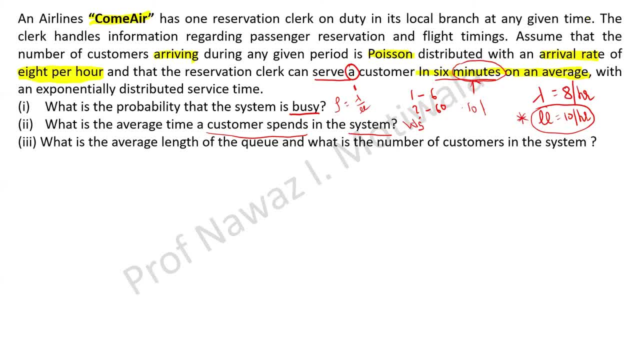 WS? Yes, it will be WS. Time is asked, meaning waiting time, or system is asked: Yes, so it will be WS. Now next, What is average length of queue? Simple is asked length of queue, So it will be length of queue LQ. 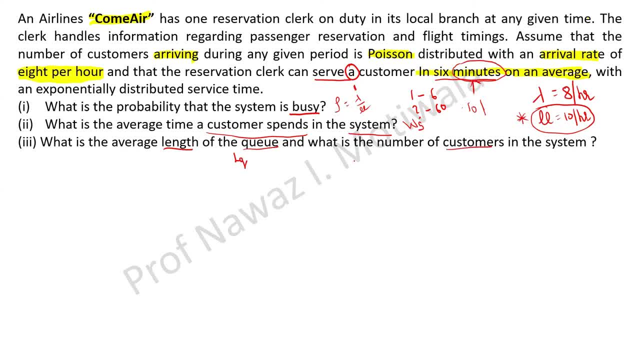 And last is: and What is the number of customers? Number? Number means length is asked of customers in the system. So what? I will write here: LS. Okay, so we need to find out. as I have written, We need to find out: lambda, WS, LQ and LS. 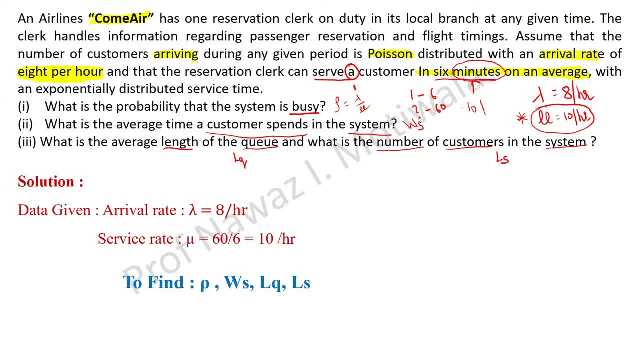 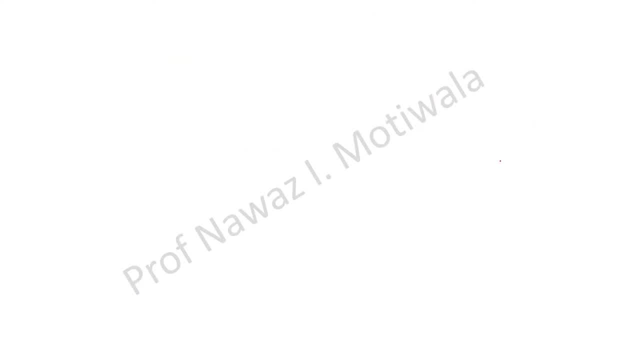 So just if you find out lambda and mu and you just scratch out what is required to be found out, Now it is becoming very easy, All the formulas I have given to you. So let us go one by one. The first formula is utilization factor, that is, rho. 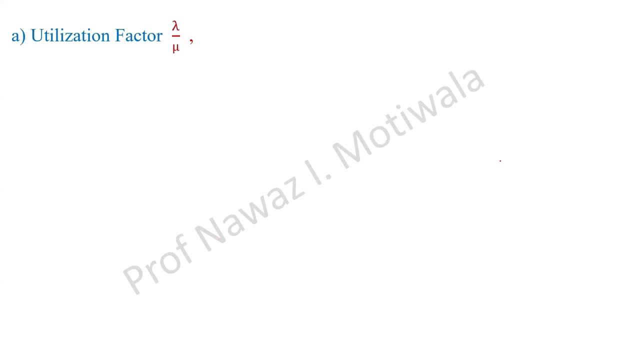 So it is lambda by mu. You have the value of lambda as 8.. You have the value of mu as 6.. So it will be lambda. Sorry, you have lambda as mu as 10. So it will be 8.. 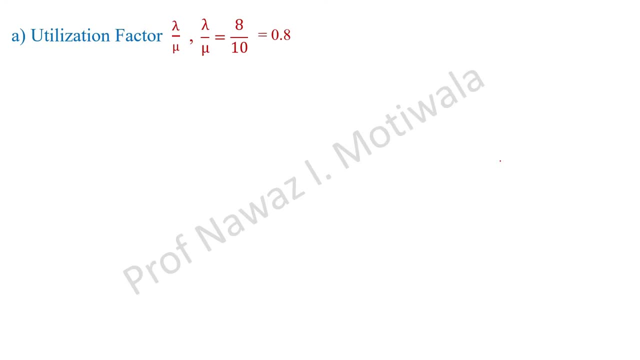 By 10, you can also write 0.8.. Okay, So now let me add one more question from my side. So let us say, if utilization factor is 0.8,, what is the probability that the system is idle? 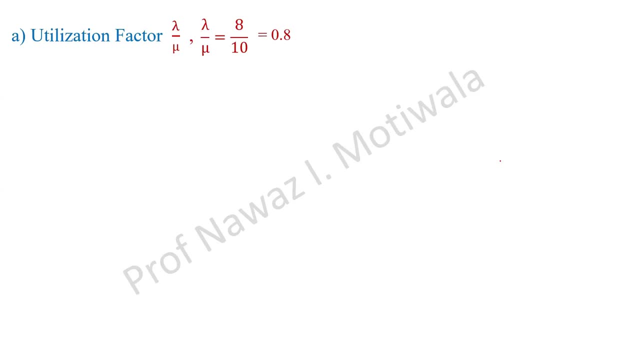 This is question from my side. Addition 0.2.. Yes, It is very simple, It will be 0.2.. Okay, Again, I will repeat this step. Utilization factor means what, How many times? How many times the system will be busy? 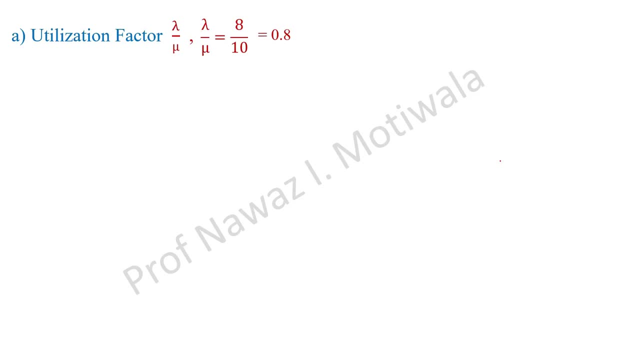 So it is giving me that 80% of time. 0.8 means 80%. It is giving me the answer that 80% of time the system will be busy. So how many times the system will be idle? It will be 100 minus 80.. 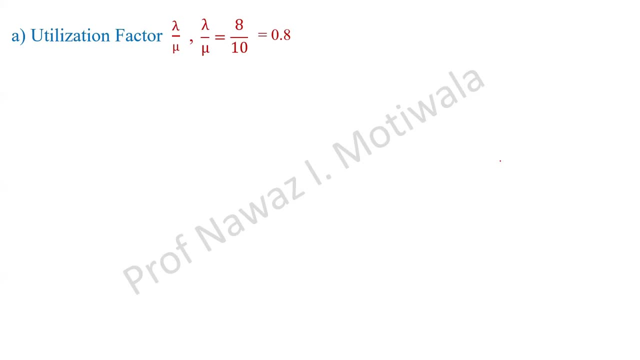 That is 20% Or I can write it 0.2.. So, anywhere you can do and you will get the same answer: 0.2 or you will get 20%. Second Second thing asked was the average number of customers in the queue. 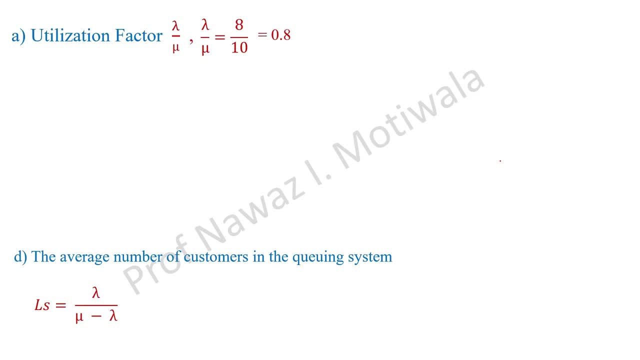 Okay, So it will be. ls is equal to lambda upon mu Minus lambda, again lambda You have. you do have suggest. I will substitute and get the answer that length of the system will be. for now, length of the system means the persons who are waiting in the queue plus the number of customers who are getting the service. 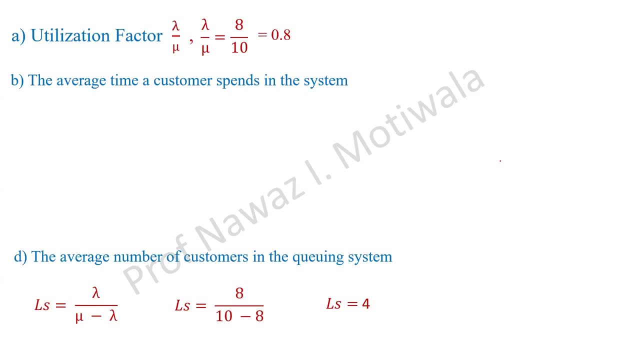 The third thing is average time a customer spends in the system. system means WS, So WS formula is one upon mu minus lambda, So it will be one upon 10 minus eight And it will be 0.5 hours. Okay. 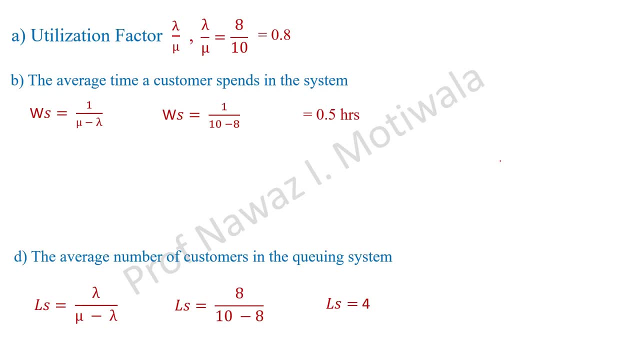 Because it is waiting time. Time will be always in hours because we have used the lambda value in hours per hour. Next, The last thing was average time of number of customers in the queue. Number of customers means lq. Lq formula is ls into lambda by mu. 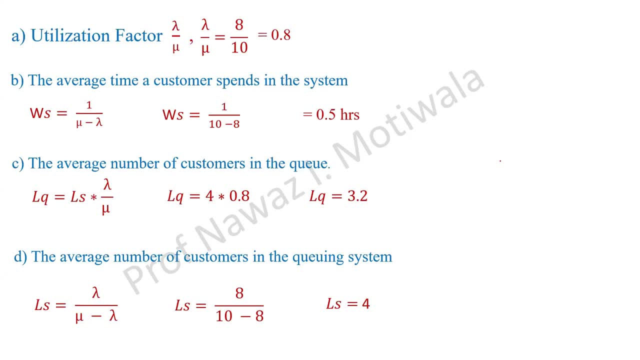 Formula will be 4 into 0.8.. And that will answer will be 3.2.. So again, Sir. So here again you emphasize on the word average. I have taken the average of all that you add up all the length of the queues at that particular time. that's why it is coming in decimals. okay, any doubts in solving the problem? so important thing was to fetch the value of lambda and fetch the value of mu and convert it into proper units. 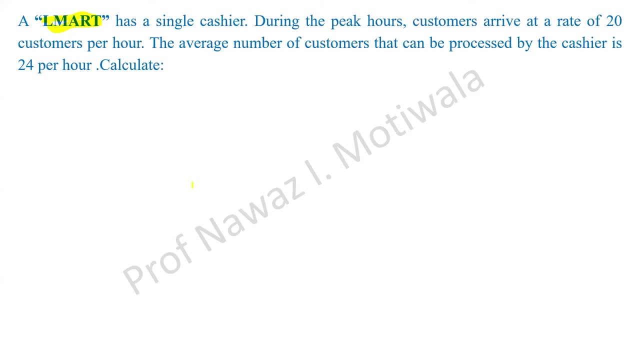 Elma. Elma has a single cashier. during the peak hour, customer arrived again, again. this is the important thing, jokes apart. during the peak hours, customer arrived at a rate of 20 customers per hour. So what can you write about this data in terms of notations? 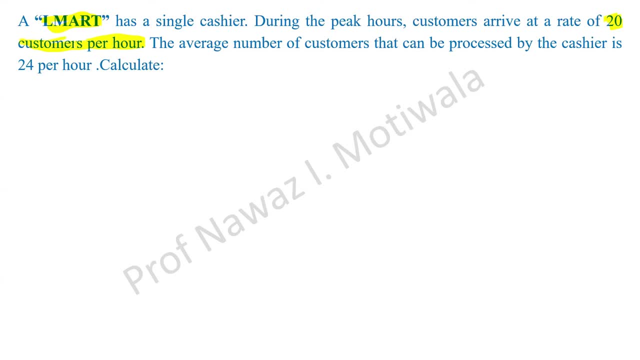 What should I write? Customer arrived both the lambda. I got 20 per hour, we both the. so no issues. directly I will write: lambda is equal to 20 per hour. Okay, The average number of customers that can be processed, processed- processed by the cashier that means he will be giving the service- is 24 per hour. 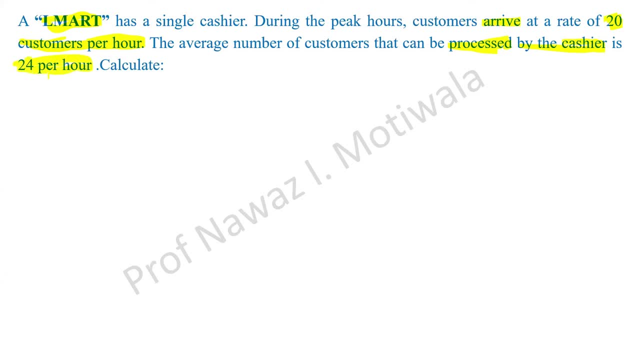 So any calculation or any conversion I require here, No, sir, No sir, Because directly it is given per hour, So, and it is service processed by the cashier, That means it is a service rate. So I will directly write: mu is equal to 24 per hour. 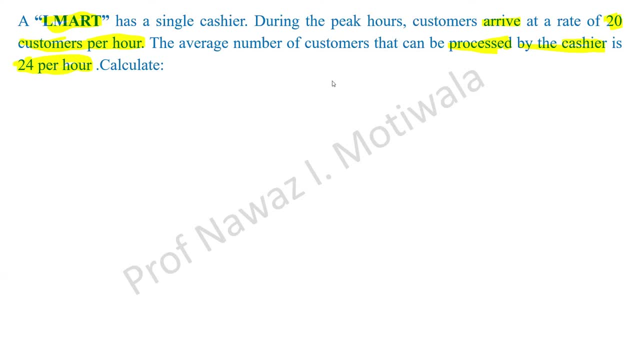 So This was a straight question wherein there is no conversion of data is required. So, as we have discussed, we will write: lambda is equal to 20 per hour And we will write: mu is equal to how much 24 per hour. 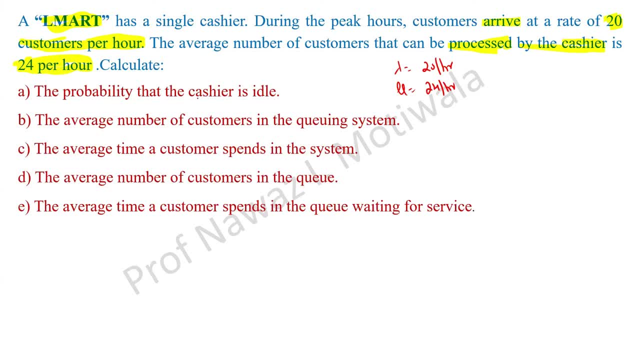 Then probably that system or the cashier is idle. So what do we need to find? Give me in terms of notation Here- I don't know P naught, Yes, The average number of customers in the queuing system. Yeah, 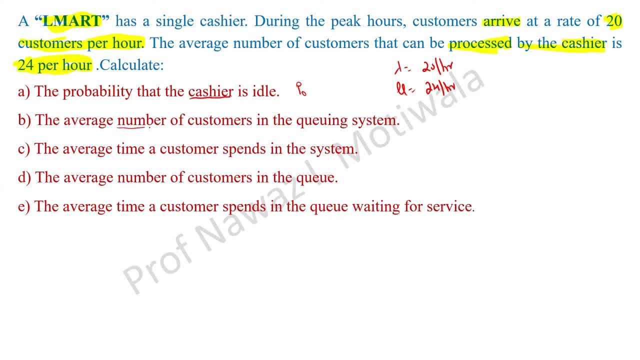 Average number number I get my stuff. Yeah, Then number means less, or your parking system will be, so it will be LS. Okay. Next, average time I'm going to have a waiting time of customers spends in the WS. Average number of customer number. 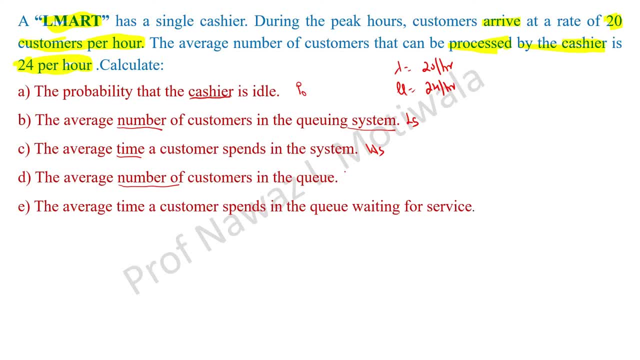 I got my stuff And customers in the queue will be at the LQ Then average time a customer spends in the queue waiting for service. waiting for service. My job WQ, waiting for service. that's why it is WQ. 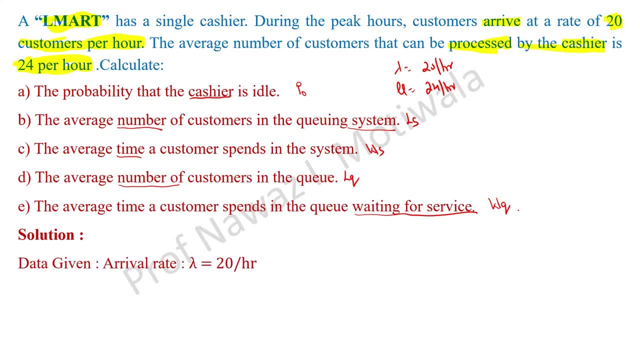 Okay, So proceeding further with the solution: Arrival late, 20 per hour, 24 hour per hour, And we have to find out, despite things, P zero, LQ, WS, L, S and WQ. Okay, Let us go one by one. 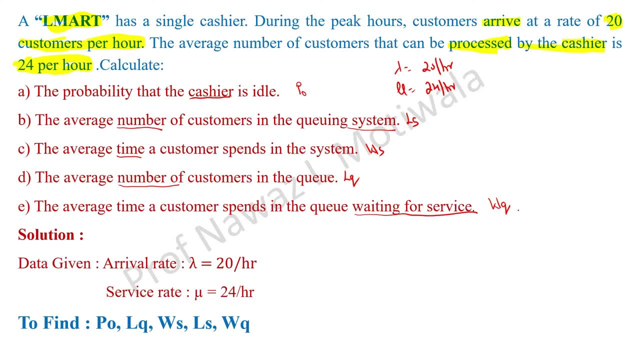 Now it's very simple problem, Just you need to apply the formula. Okay, So to find out? I don't think to find out, I don't think we cannot go directly. first, We need to find out what is utilization factor. So utilization factor is lambda by new lambda. 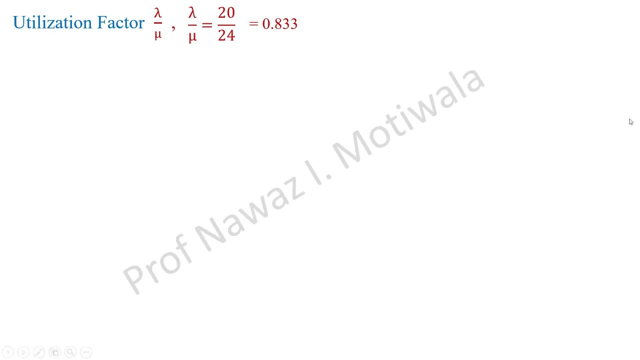 We have 20 new, we have 24.. So I will get that answer as how much? we are getting 0.833.. So 0.833 means 83.3% of time. The system will be busy, So how much time it will be idle? 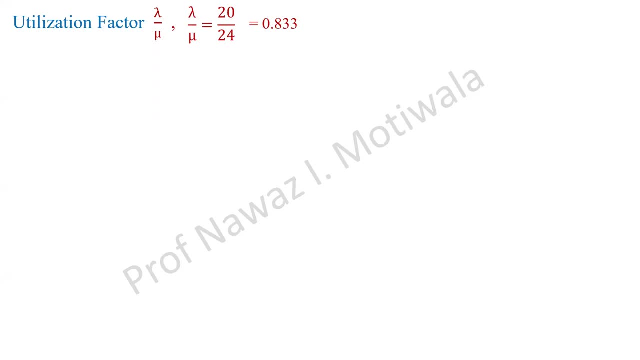 It will be simple: one minus 0.8.. That means 0.1, seven. That means 17% Of time the cashier will be idle. So you are getting 0.1, 6, 6,, 6, 7.. 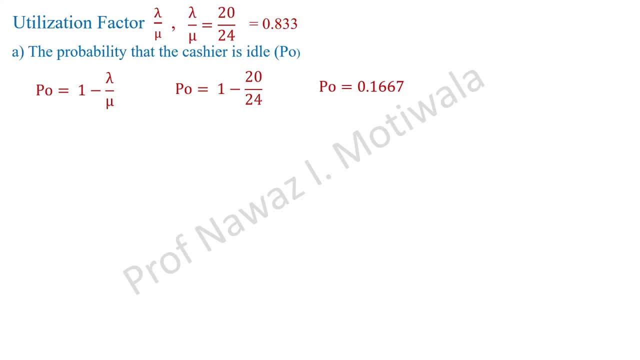 Exactly. Second thing which was asked in the question was average number of customers in the queuing system. So number of customers in the queuing system will be LS lambda upon you minus lambda, So it will be 20 upon 24 minus 20. answer will be five, 20 upon 4, 20 upon four.